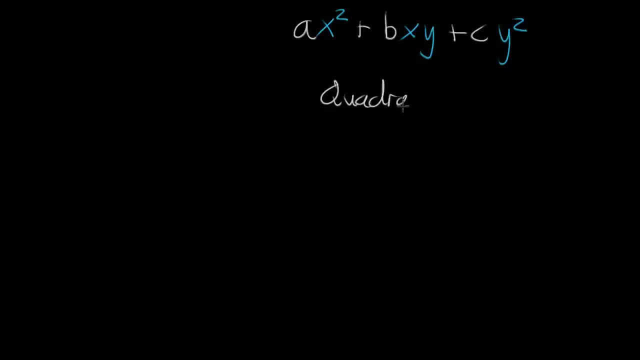 It's called a quadratic form, Quadratic form, And that always threw me off. I always kind of was like: what does form mean? You know, I know what a quadratic expression is, and quadratic typically means something is squared or you have two variables. but why do they call it a form? 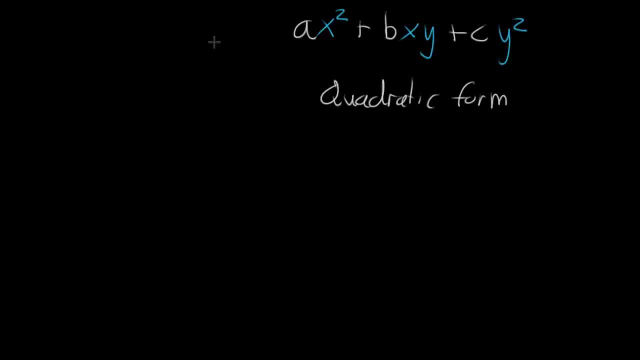 And basically it just means that the only things in here are quadratic. You know, it's not the case that you have like an x term sitting on its own or like a constant out here, like two, and you're adding all of those together. 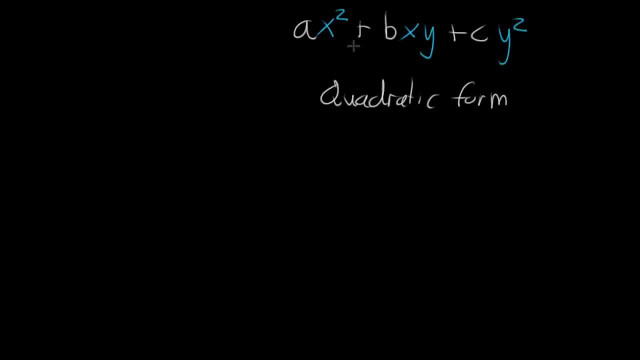 Instead it's just: you have purely quadratic terms, But of course mathematicians don't want to call it just a purely quadratic form. Instead, they have to give a fancy name to things so that it seems more intimidating than it needs to be. 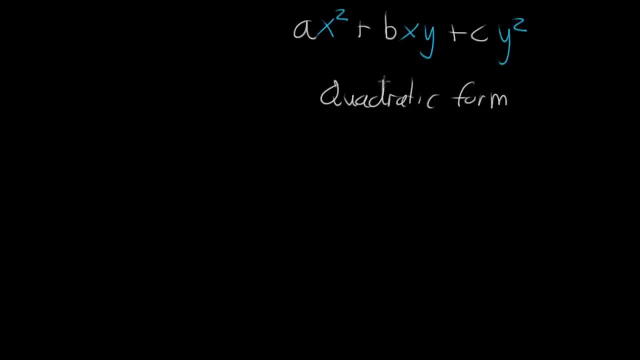 But anyway. so we have a quadratic form and the question is, how can we express this in a vectorized sense? And for analogy, let's think about linear terms where, let's say, you have a times x plus b times y? 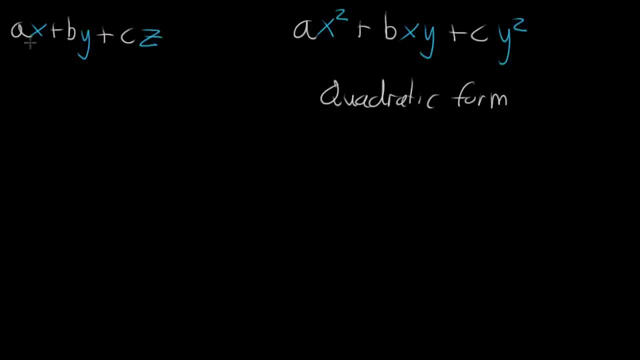 and I'll throw another variable in there, another constant times, another variable z. If you see something like this, where every variable is just being multiplied by a constant and then you add terms like that to each other, we can express this nicely with vectors. 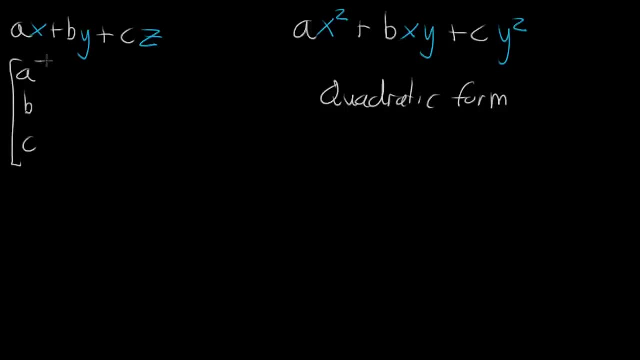 where you pile all of the constants into their own vector, a vector containing a, b and c, and you imagine the dot product between that and a vector that contains all of the variable components x, y and z, And the convenience here is: then you can have. 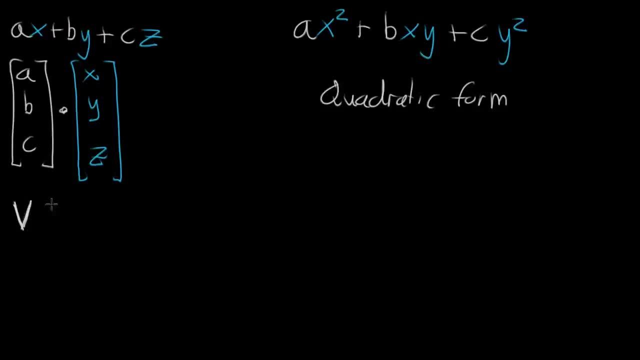 just a symbol like a v, let's say, which represents this whole constant vector, and then you can write down: take the dot product between that and then have another symbol, maybe a bold-faced x, which represents a vector that contains 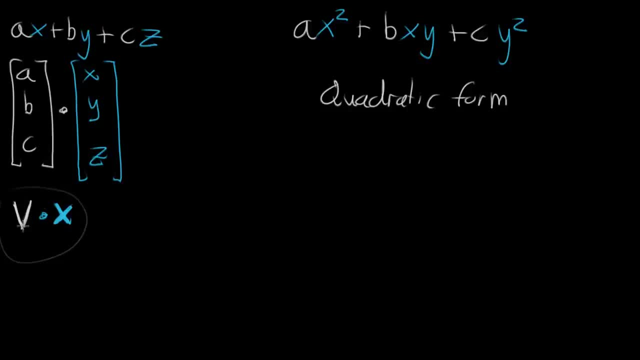 all of the variables and this way your notation just kind of looks like a constant times a variable, just like in the single variable world, when you have a constant number times a variable number. it's kind of like taking a constant vector times a variable vector. 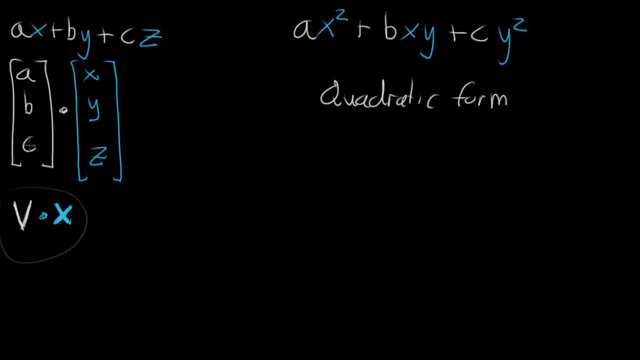 And the importance of writing things down like this is that v could be a vector that contains not just three numbers, but like 100 numbers, and then x would have 100 corresponding variables, and the notation doesn't become any more complicated. It's generalizable to higher dimensions. 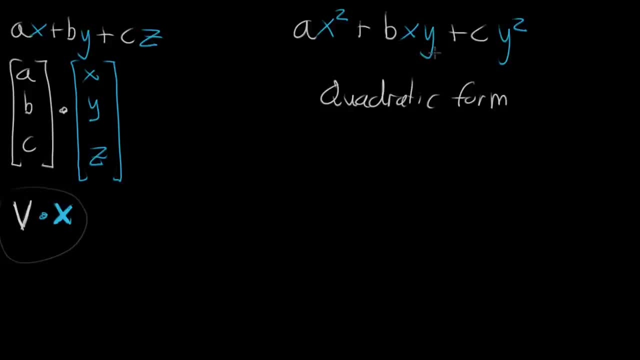 So the question is, can we do something similar like that with our quadratic form? Because you can imagine, let's say, we started introducing the variable z, Then you would have to have some other term, you know some other constant times, the xz quadratic term. 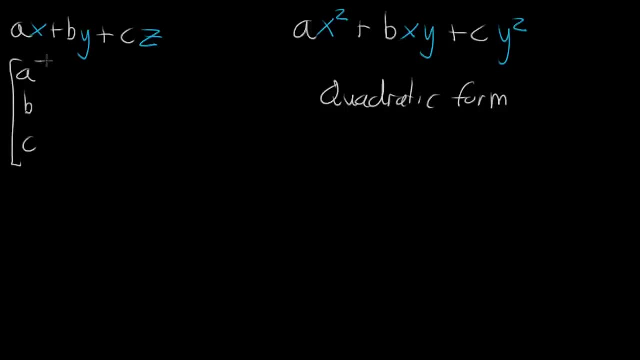 where you pile all of the constants into their own vector, a vector containing a, b and c, and you imagine the dot product between that and a vector that contains all of the variable components x, y and z, And the convenience here is: then you can have. 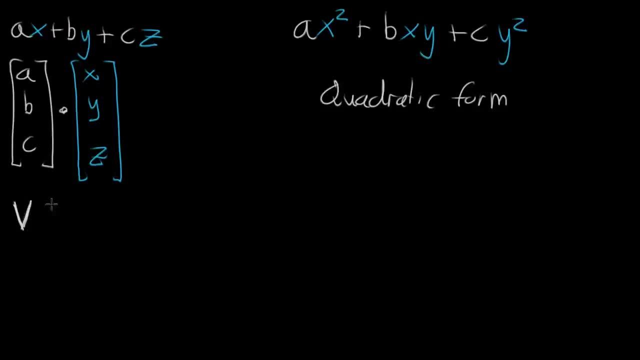 just a symbol like a v, let's say, which represents this whole constant vector, and then you can write down: take the dot product between that and then have another symbol, maybe a bold-faced x, which represents a vector that contains 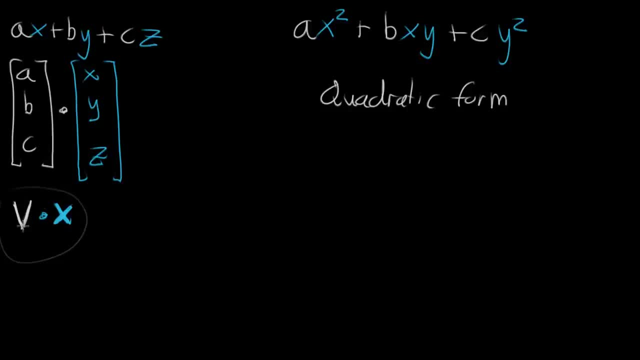 all of the variables and this way your notation just kind of looks like a constant times a variable, just like in the single variable world, when you have a constant number times a variable number. it's kind of like taking a constant vector times a variable vector. 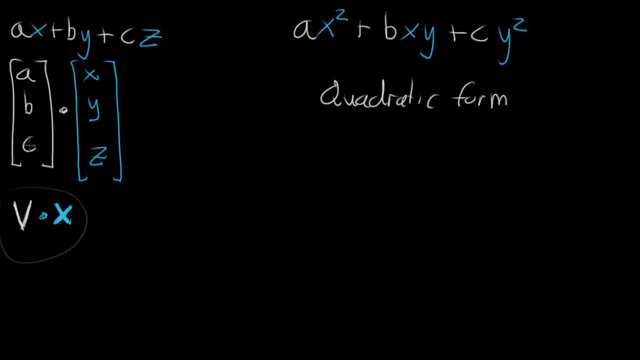 And the importance of writing things down like this is that v could be a vector that contains not just three numbers, but like 100 numbers, and then x would have 100 corresponding variables, and the notation doesn't become any more complicated. It's generalizable to higher dimensions. 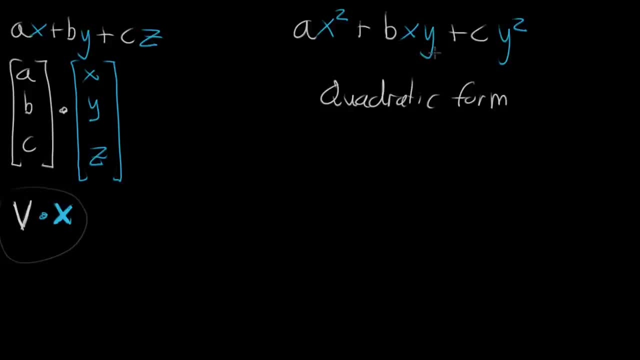 So the question is, can we do something similar like that with our quadratic form? Because you can imagine, let's say, we started introducing the variable z, Then you would have to have some other term, you know some other constant times, the xz quadratic term. 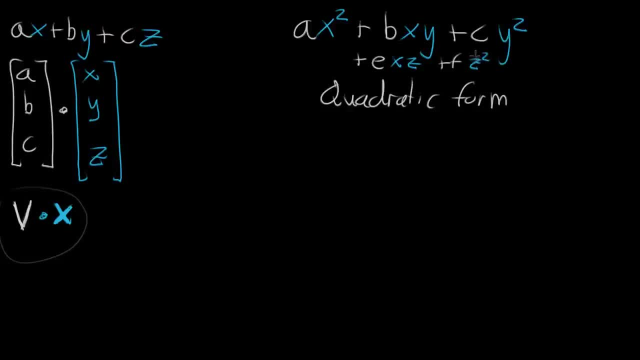 and then some other constant times, the z squared quadratic term, and another one for the yz quadratic term, and it would get out of hand. and as soon as you start introducing things like 100 variables, it would get seriously out of hand. 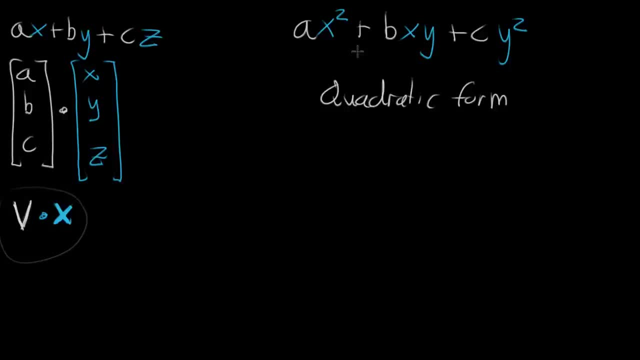 because there's a lot of different quadratic terms. So we want a nice way to express this And I'm just gonna kind of show you how we do it and then we'll work it through to see why it makes sense. So usually, instead of thinking of b times, xy. 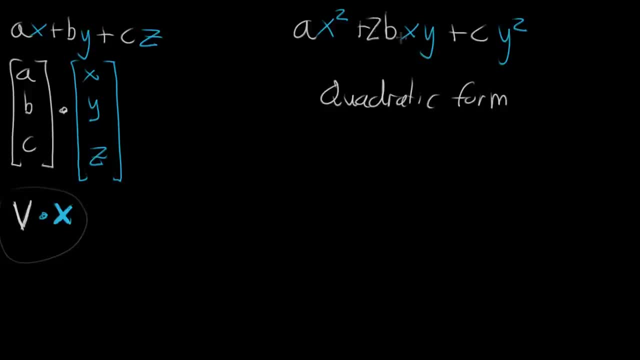 we actually think of this as two times, some constant times, xy, And this, of course, doesn't make a difference. You would just change what b represents. But you'll see why it's more convenient to write it this way in just a moment. 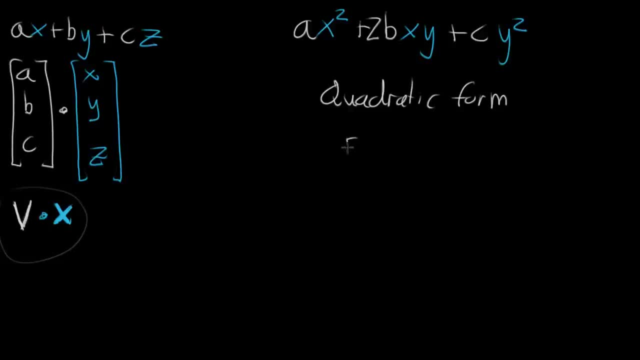 So the vectorized way to describe a quadratic form like this is to take a matrix, a, two by two matrix, since this is two dimensions, where a and c are on the diagonal and then b is on the other diagonal, And we always think of these as being symmetric matrices. 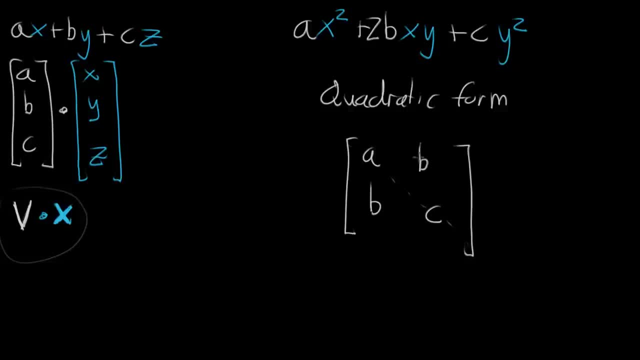 So if you imagine kind of reflecting the whole matrix about this line, you'll get the same numbers. So it's important that we have that kind of symmetry. And now what you do is you multiply the vector, the variable vector, that's got xy. 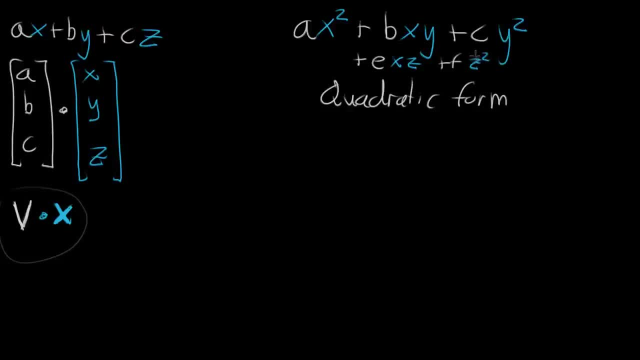 and then some other constant times, the z squared quadratic term, and another one for the yz quadratic term, and it would get out of hand. and as soon as you start introducing things like 100 variables, it would get seriously out of hand. 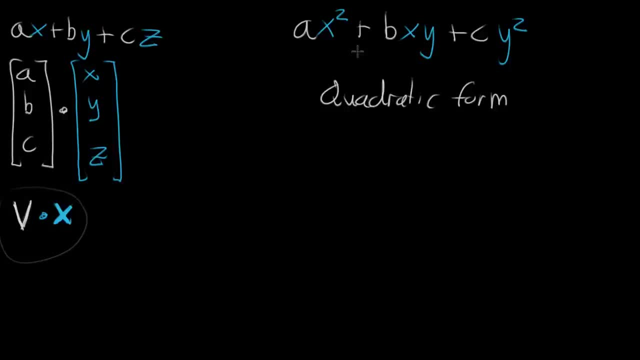 because there's a lot of different quadratic terms. So we want a nice way to express this And I'm just gonna kind of show you how we do it and then we'll work it through to see why it makes sense. So usually, instead of thinking of b times, xy. 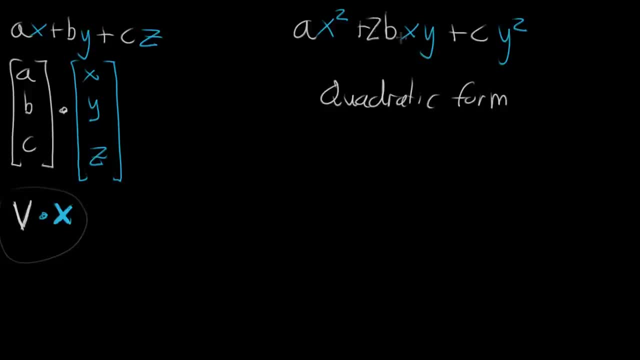 we actually think of this as two times, some constant times, xy, And this, of course, doesn't make a difference. You would just change what b represents. But you'll see why it's more convenient to write it this way in just a moment. 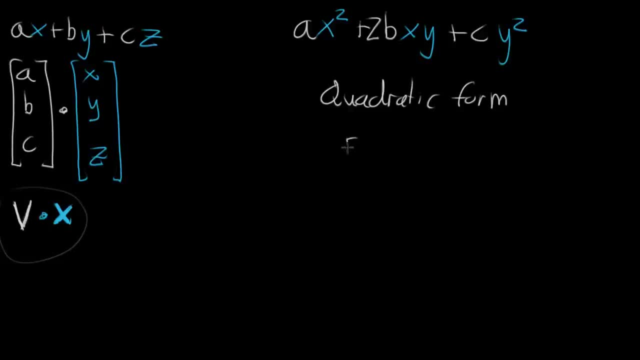 So the vectorized way to describe a quadratic form like this is to take a matrix, a, two by two matrix, since this is two dimensions, where a and c are on the diagonal and then b is on the other diagonal, And we always think of these as being symmetric matrices. 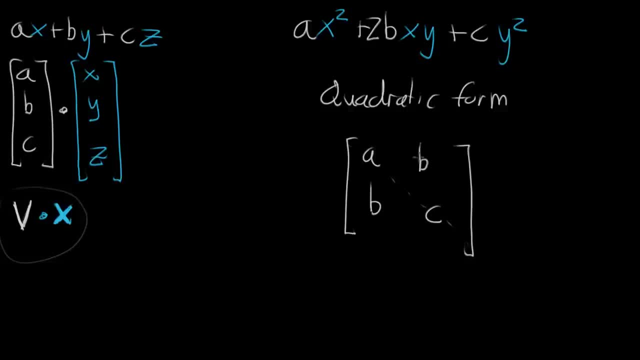 So if you imagine kind of reflecting the whole matrix about this line, you'll get the same numbers. So it's important that we have that kind of symmetry. And now what you do is you multiply the vector, the variable vector, that's got xy. 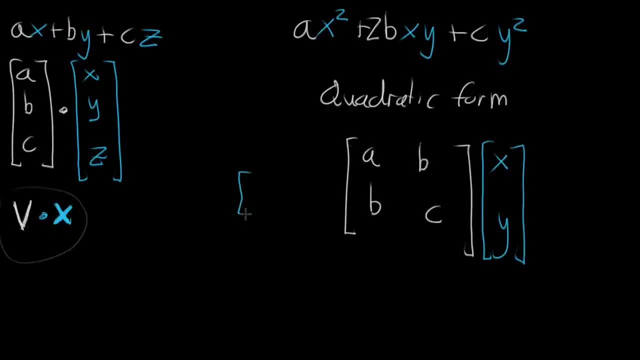 on the right side of this matrix and then you multiply it again, but you kind of you turn it on its side. So instead of being a vertical vector, you transpose it to being a horizontal vector on the other side, And this is a little bit analogous to you know. 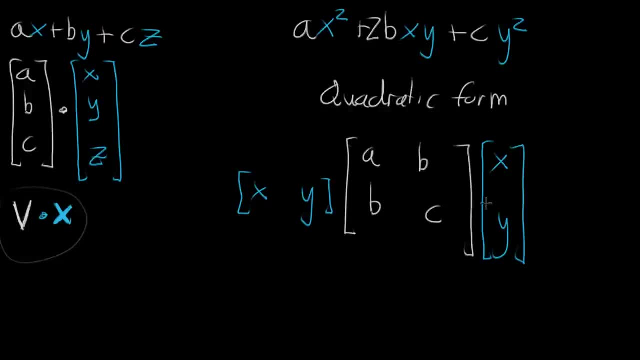 having two variables multiplied in. You have two vectors multiplied in, but on either side, And this is a good point. by the way, if you are uncomfortable with matrix multiplication, to maybe pause the video, go find the videos about matrix multiplication and kind of refresh or learn about that. 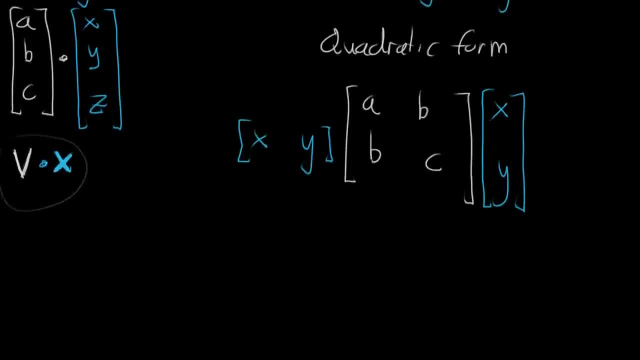 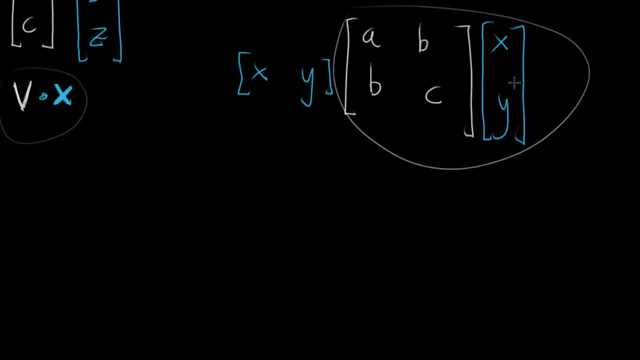 Because, moving forward, I'm just going to assume that it's something you're familiar with. So going about computing this, first, let's tackle this right multiplication. here We have a matrix multiplied by a vector. Well, the first component that we get, 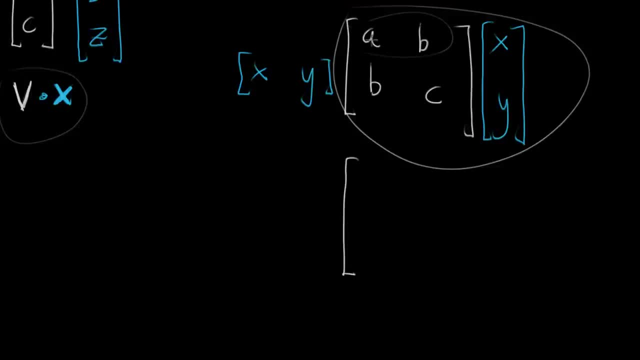 we're going to multiply the top row by each corresponding term in the vector, So it'll be a times x, a times x plus b times y plus b times that second term term, y, And then similarly for the bottom term. 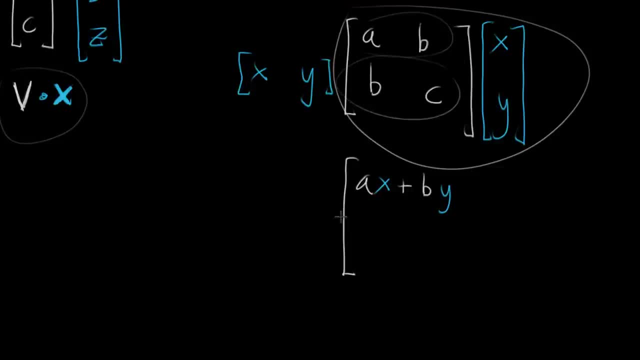 we'll take the bottom row and multiply the corresponding terms, So b times x, b times x, plus c times y, c times y. So that's what it looks like when we do that right multiplication. And of course we've got to keep our transposed vector. 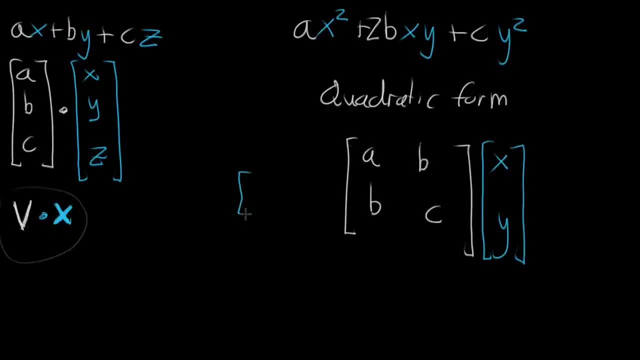 on the right side of this matrix and then you multiply it again, but you kind of you turn it on its side. So instead of being a vertical vector, you transpose it to being a horizontal vector on the other side, And this is a little bit analogous to you know. 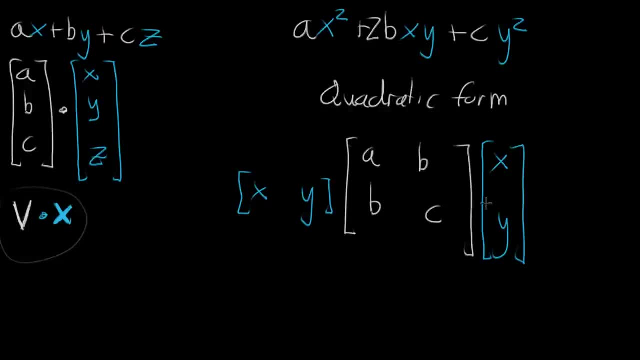 having two variables multiplied in. You have two vectors multiplied in, but on either side, And this is a good point. by the way, if you are uncomfortable with matrix multiplication, to maybe pause the video, go find the videos about matrix multiplication and kind of refresh or learn about that. 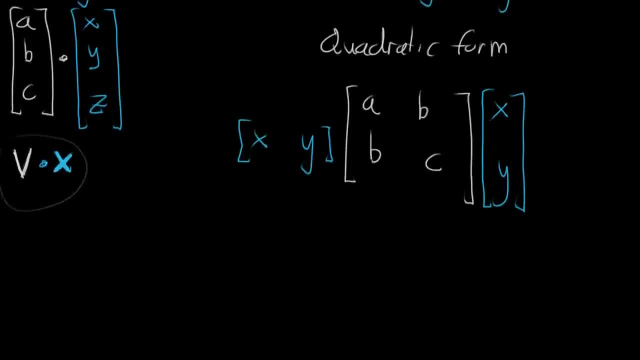 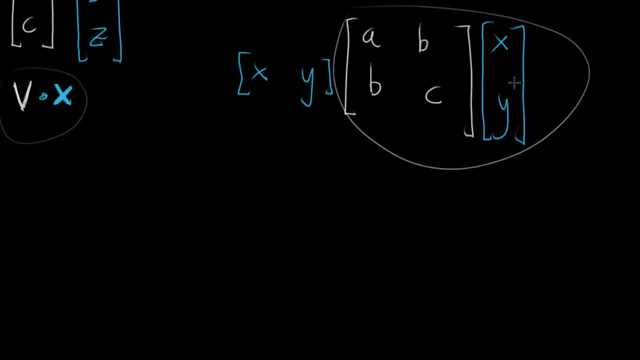 Because, moving forward, I'm just going to assume that it's something you're familiar with. So going about computing this, first, let's tackle this right multiplication. here We have a matrix multiplied by a vector. Well, the first component that we get, 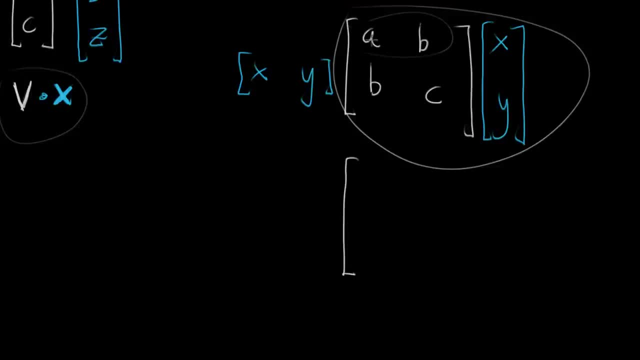 we're going to multiply the top row by each corresponding term in the vector, So it'll be a times x, a times x plus b times y plus b times that second term term, y, And then similarly for the bottom term. 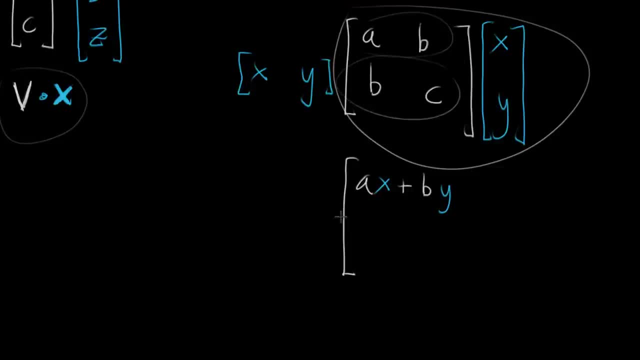 we'll take the bottom row and multiply the corresponding terms, So b times x, b times x, plus c times y, c times y. So that's what it looks like when we do that right multiplication. And of course we've got to keep our transposed vector. 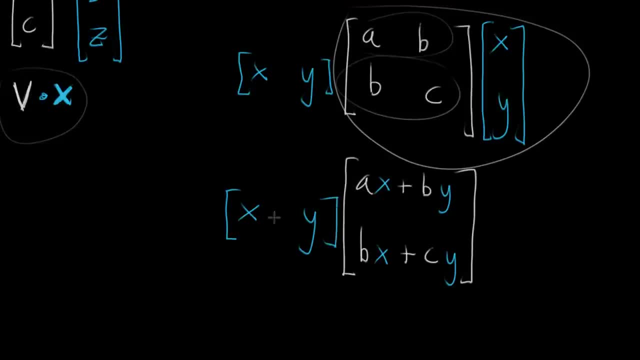 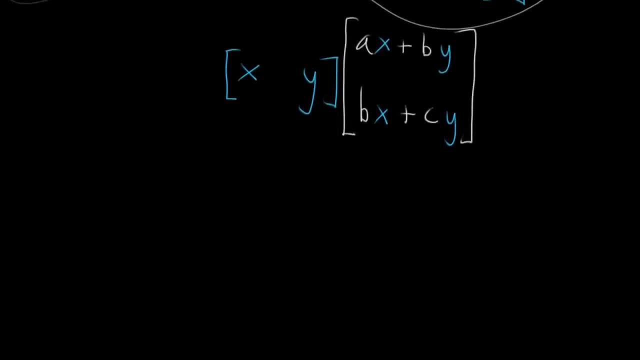 over there on the left side. So now we have, this is just a two by one vector. now This is a one by two. You could think of it as a two by one vector or a one by two matrix. But now when we multiply these guys, 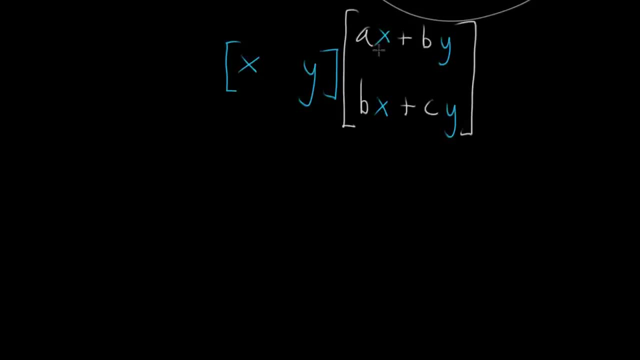 you just kind of line up the corresponding terms, You'll have x multiplied by that entire top expression, So x multiplied by ax plus by, Ax plus by, And then we add that to the second term, y multiplied by the second term of this guy. 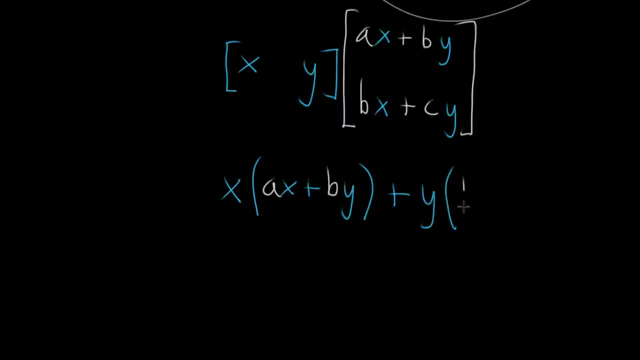 which is bx plus cy, So y multiplied by bx plus cy, So y multiplied by bx plus cy. And all of these are numbers so we can simplify it Once we start distributing. the first term is x times a times x, So that's ax squared. 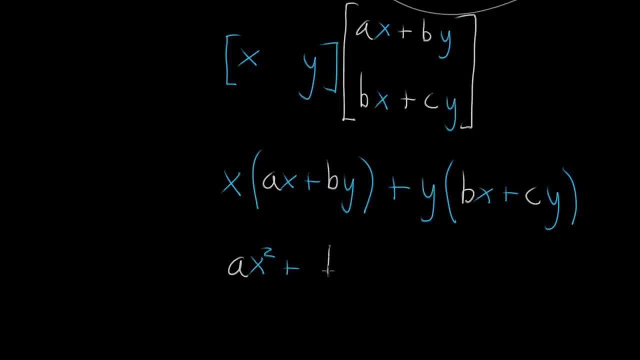 And then the next term is x times b times y, So that's b times xy. Over here we have y times b times x, So that's the same thing as b times xy. So that's kind of why we have, why it's convenient to write a two there. 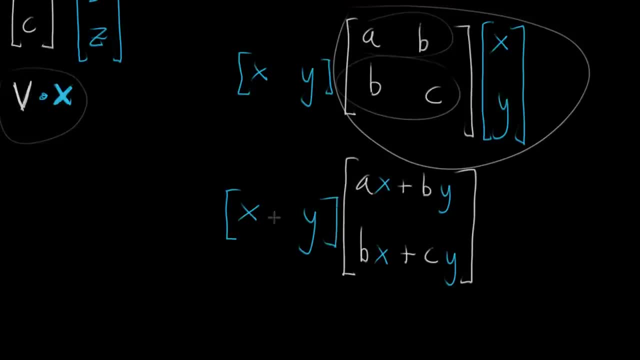 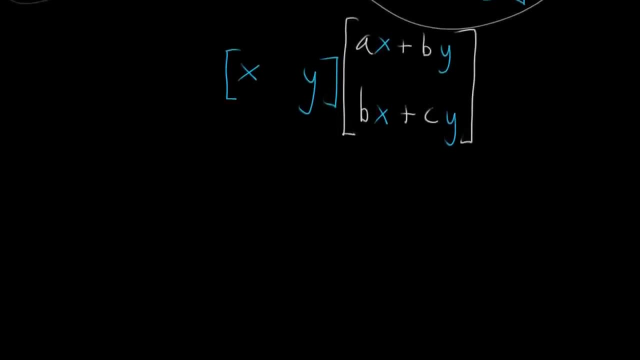 over there on the right, on the left side. So now we have, this is just a two by one vector now and this is a one by two. You could think of it as a two by one vector or a one by two matrix. 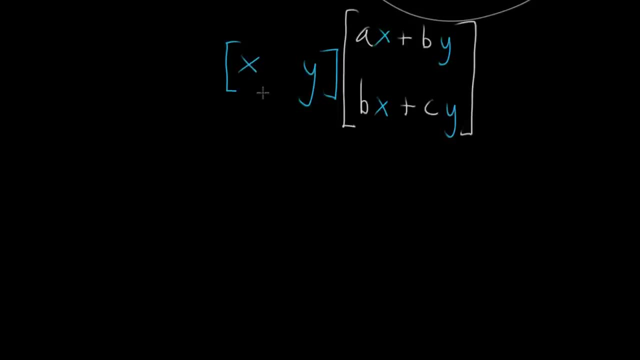 But now when we multiply these guys, you just kind of line up the corresponding terms- You'll have x multiplied by that entire top expression, So x multiplied by ax plus by, Ax plus by, And then we add that to the second term, y. 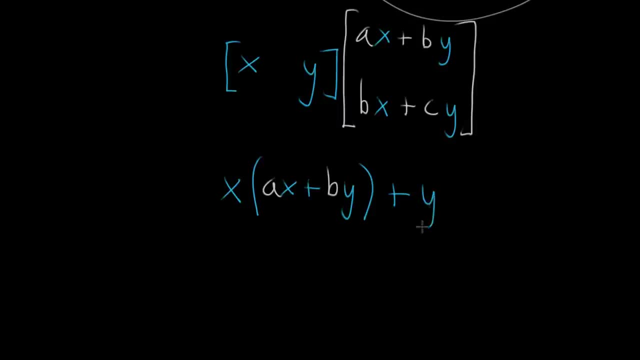 multiplied by the second term of this guy, which is bx plus cy, So y multiplied by bx plus cy, So y multiplied by bx plus cy. And all of these are numbers so we can simplify it Once we start distributing. the first term is x times a times x. 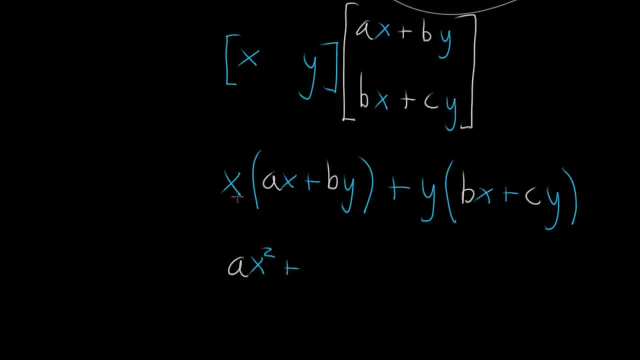 So that's ax squared. And then the next term is x times b times y, So that's b times xy. Over here we have y times b times x, So that's the same thing as b times xy. So that's kind of why we have 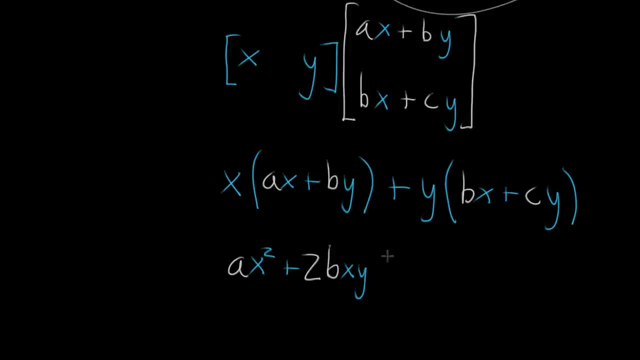 why it's convenient to write a two there, because that naturally comes out of our expansion. And then the last term is y times c times y, So that's cy squared. So we get back the original quadratic form that we were shooting for. 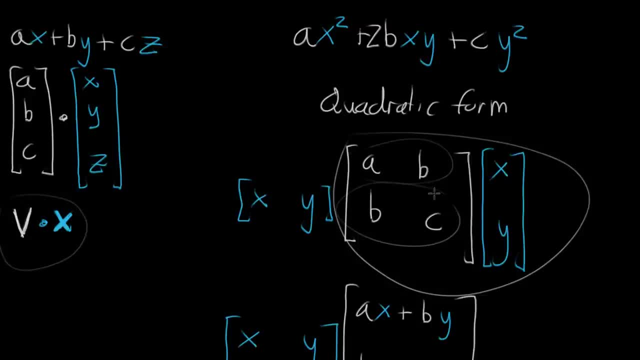 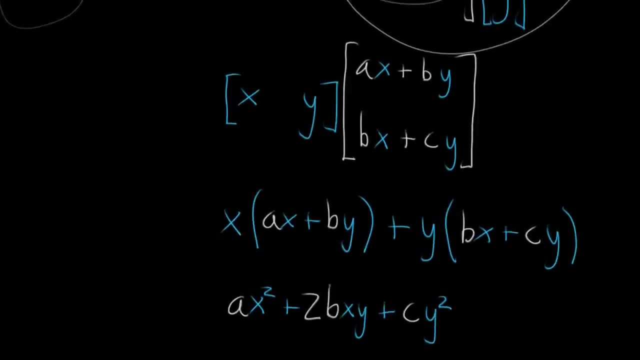 You know, ax squared plus 2bxy plus cy squared. That's how this entire term expands. As you kind of work it through, you end up with the same quadratic expression. Now, the convenience of this quadratic form being written with a matrix like this: 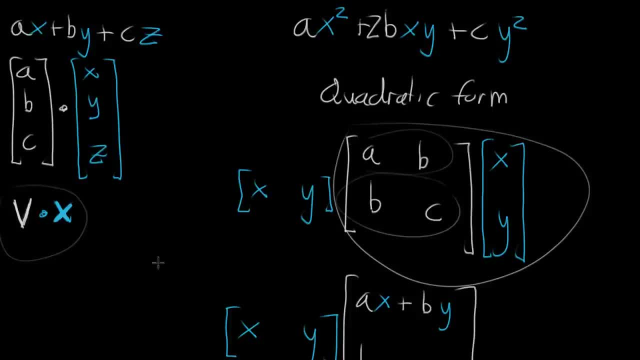 is that we can write this more abstractly And instead of writing the whole matrix M, you could just let a letter like M represent that whole matrix And then take the vector that represents the variable, maybe like a bold-faced x, and you would multiply it on the right. 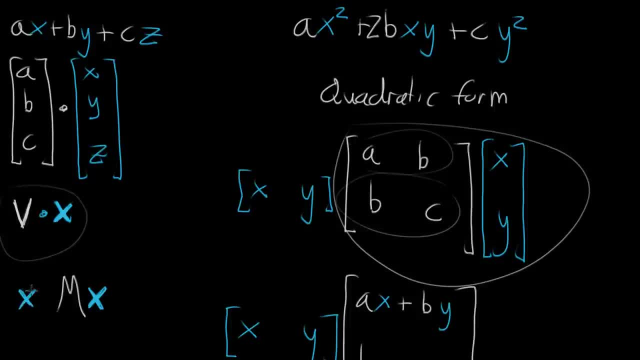 And then you transpose it and multiply it on the left. So typically you denote that by putting a little t as a superscript. So x transposed, multiplied by the matrix from the left And this expression. this is what a quadratic form looks like in vectorized form. 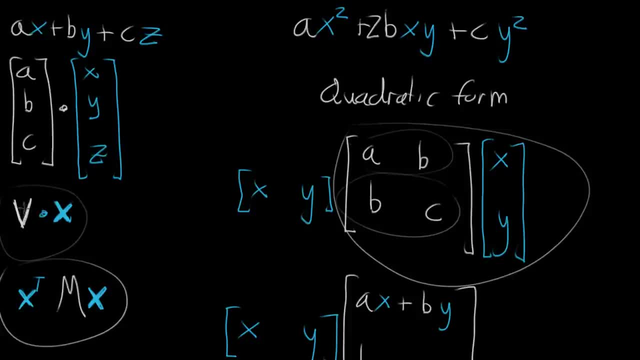 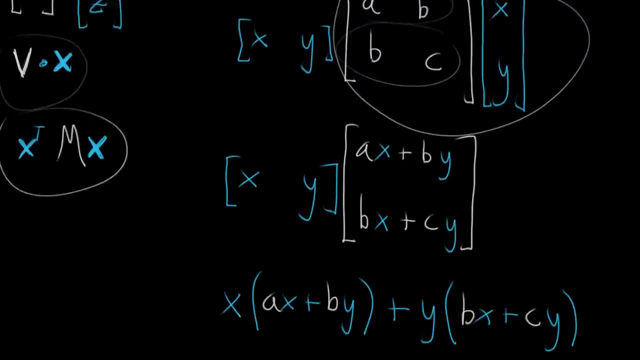 And the convenience is the same as it was in the linear case. Just like v could represent something that had 100 different numbers in it and x would have 100 different constants, you could do something similar here, where you can write that same expression. 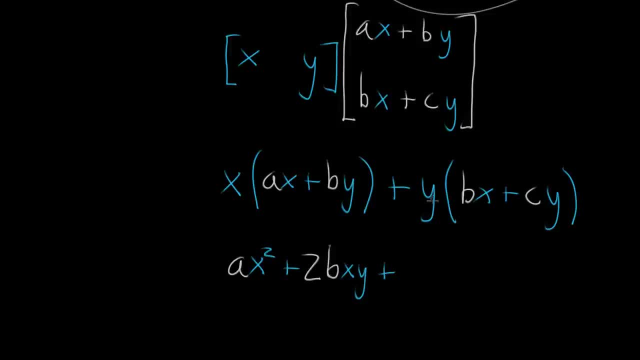 because that naturally comes out of our expansion. And then the last term is y times c times y, So that's c times x, So that's 2bxy squared. So we get back the original quadratic form that we were shooting for. 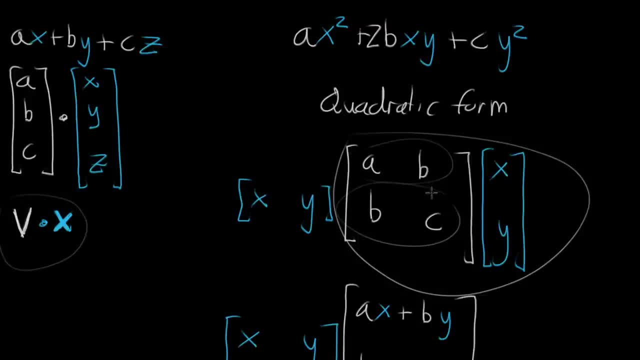 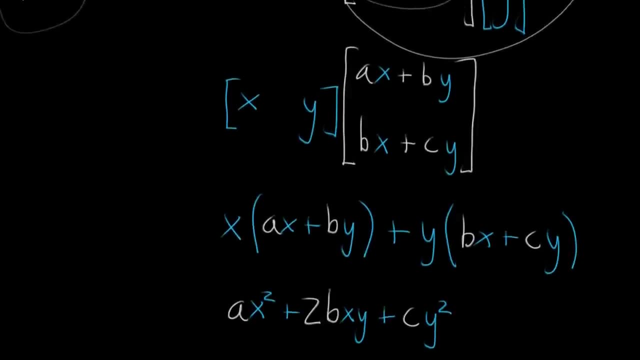 You know, ax squared plus 2bxy plus cy squared. That's how this entire term expands. As you kind of work it through, you end up with the same quadratic expression. Now, the convenience of this quadratic form being written with a matrix like this: 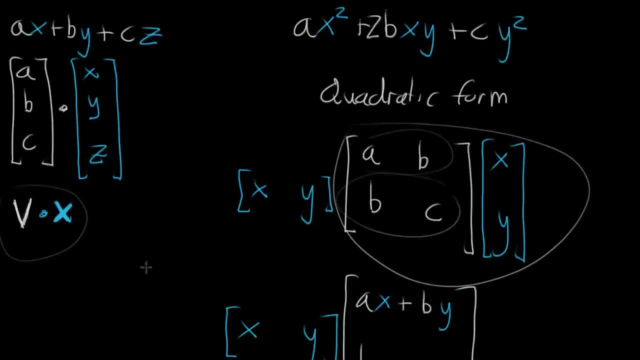 is that we can write this more abstractly, And instead of writing the whole matrix in, you could just let a letter like m represent that whole matrix And then take the vector that represents the variable, maybe like a bold-faced x, and you would multiply it on the right. 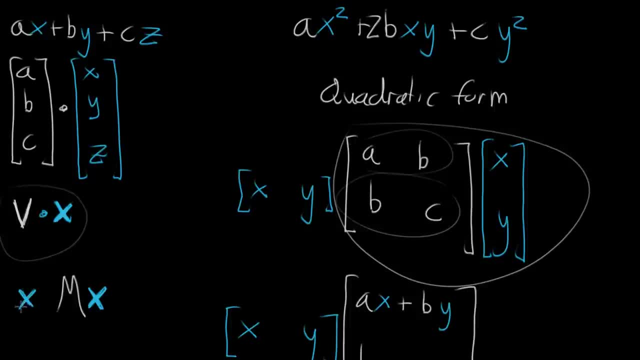 And then you transpose it and multiply it on the left. So typically you denote that by putting a little t as a superscript. So x transposed, multiplied by the matrix from the left And this expression. this is what a quadratic form looks like in vectorized form. 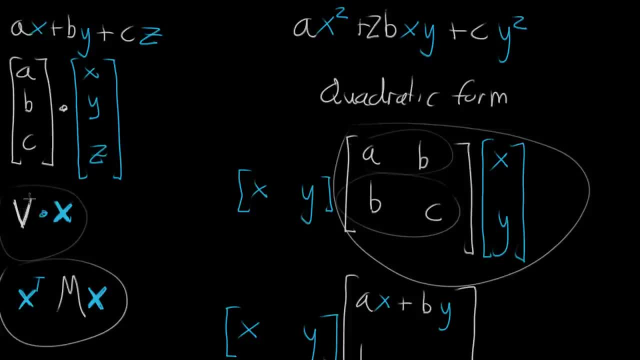 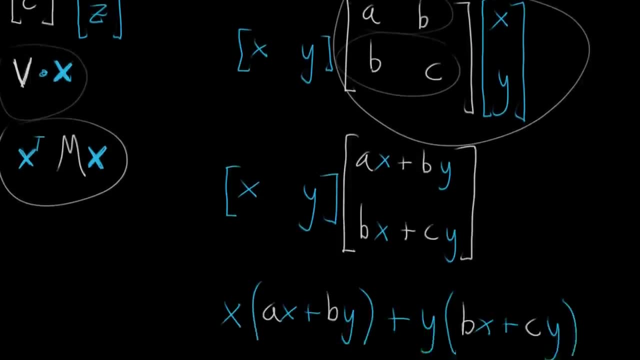 And the convenience is the same as it was in the linear case. Just like v could represent something that had 100 different numbers in it and x would have 100 different constants, you could do something similar here, where you can write that same expression. 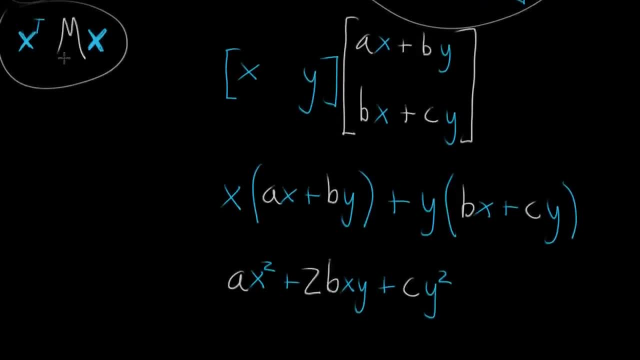 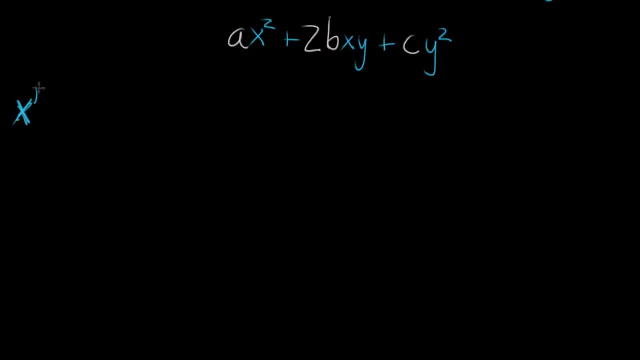 even if the matrix m is super huge, Let's just see what this would look like in a three-dimensional circumstance. So actually I'll need more room, So I'll go down even further. So we have x transposed, multiplied by the matrix. 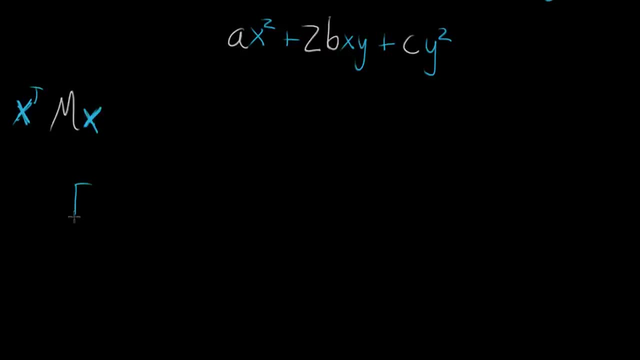 multiplied by x, bold-faced x, And let's say instead: this represented: you know, you have x, then y, then z, our transposed vector, And then our matrix. our matrix, let's say it was a, b. 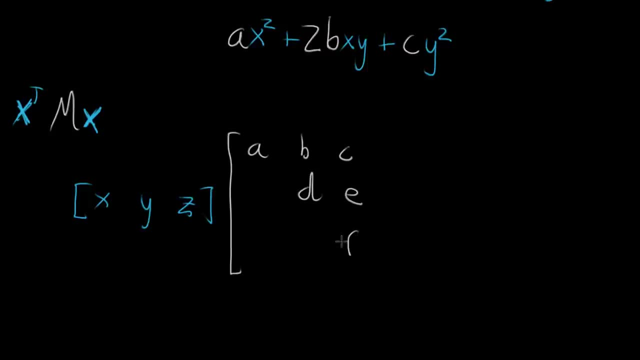 c, d, e, f, and because it needs to be symmetric, whatever term is in this spot here needs to be the same as over here, kind of when you reflected about that diagonal. Similarly, c, that's gonna be the same term here. 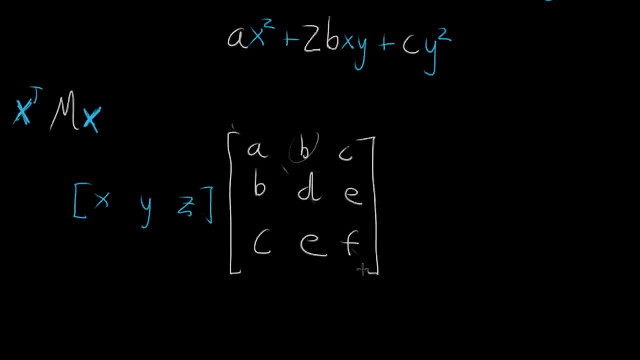 and e would be over here. So there's only really six free terms that you have, but it fills up this entire matrix. And then on the right side we would multiply that by x, y, z. Now, I won't work it out in this video. 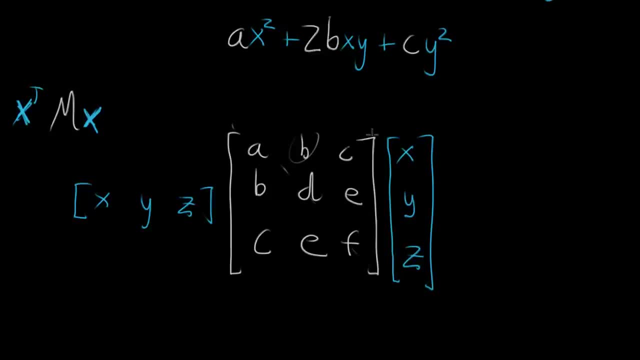 but you can imagine actually multiplying this matrix by this vector and then multiplying the corresponding vector that you get by this transposed vector and you'll get some kind of quadratic form with three variables, And the point is you'll get a very complicated one.